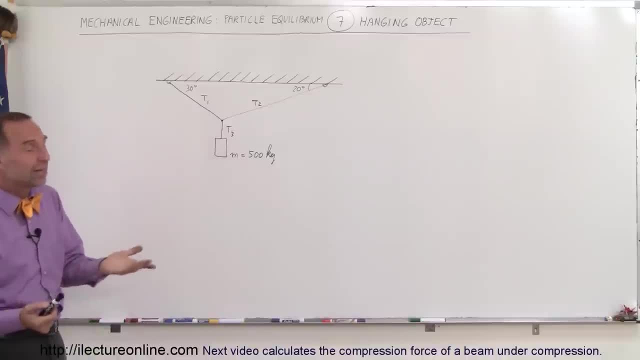 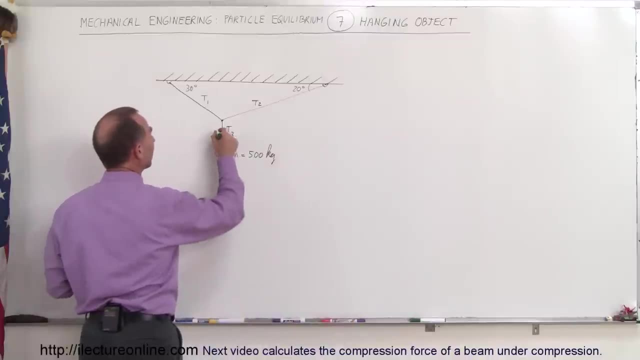 the three cables. Of course, to find the tension in cable three is fairly easy, because if we draw a free body diagram of this right here- and let me go ahead and do that- You can see that the only two forces acting on this object right here is simply the tension pulling it up and, of course, 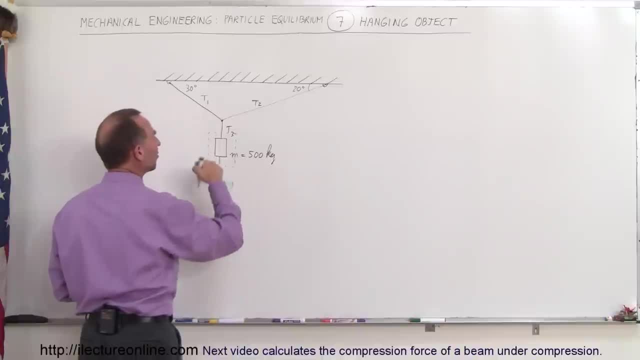 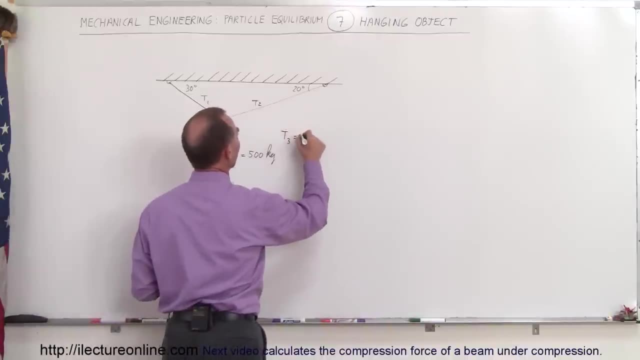 then the force of gravity pulling it down, mg, Which means that in this case tension three must equal mg, which makes it easy, and we can then write that t sub 3 is equal to mg And therefore t sub 3 is equal to the mass of the object, which is 500 kilograms times acceleration due to. gravity zero degrees. This we know. the t sub 3, we know that gave us some weight And so we have d squared and we know that the mass of the object, which is 500 kilograms times acceleration due to gravity zero degrees, If n is equal to the mass of the object, right and that is m, and Try the trial and 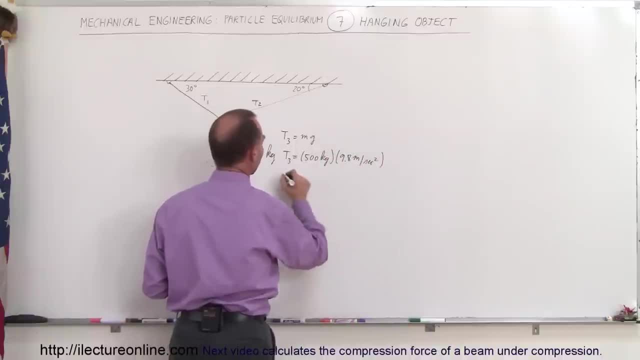 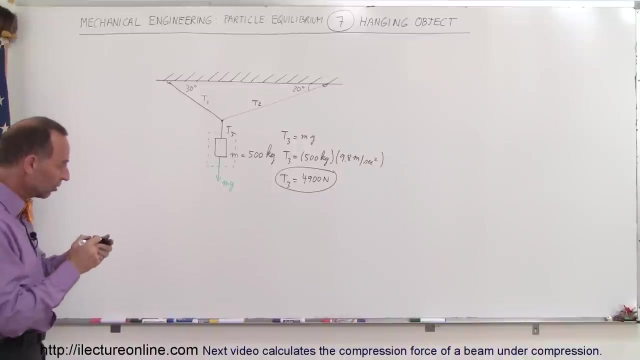 which is 9.8 meters per second squared, and that gives us tension 3 to be equal to that would be 4900 Newtons. all right, so that allows us to find tension 3, but to find tension 1 and tension 2, that is a little bit more. 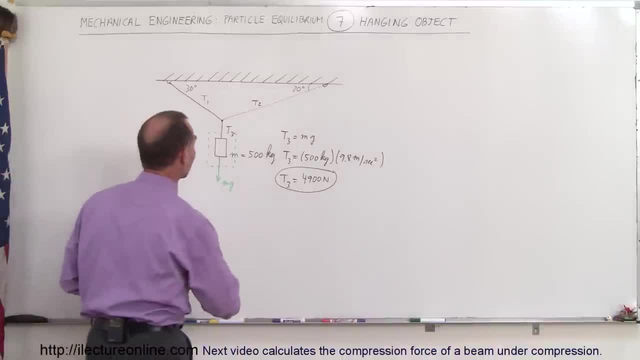 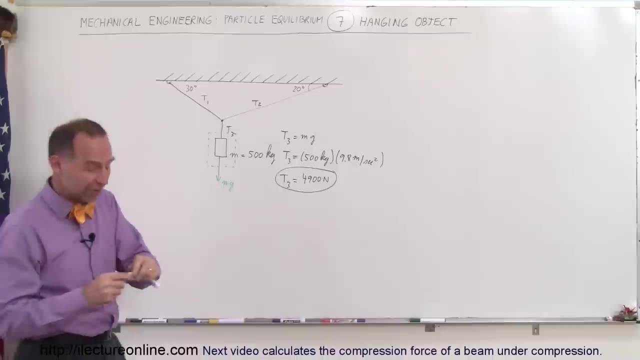 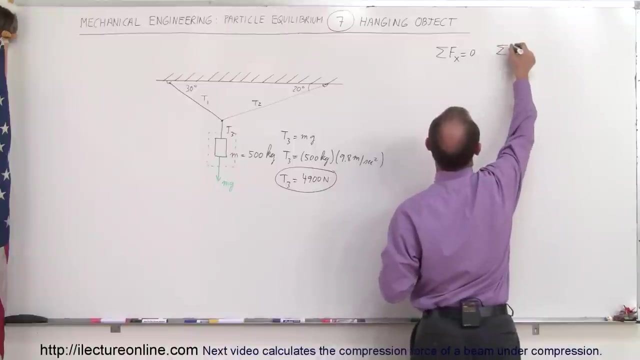 challenging. for that we need to find the two components of each of the forces, because, again, it's a situation, it's an, it's a problem where everything is in equilibrium. and if everything is in equilibrium, we know that the sum of the forces in the x-direction must add up to 0 and the sum of the forces in the 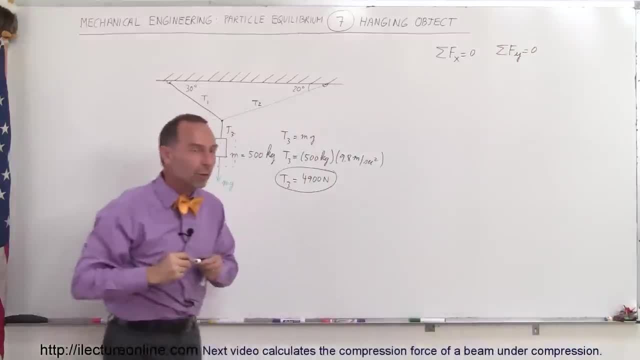 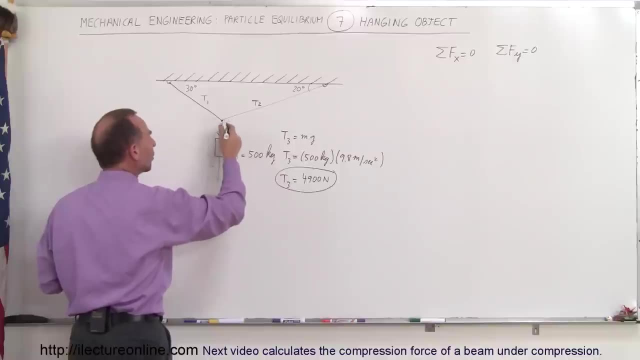 y-direction must add up to 0, which means we need to find the X&Y components of each of the forces there. now notice: of course tension 3 will be acting in a downward direction. there's only one component, so we don't have to divide. 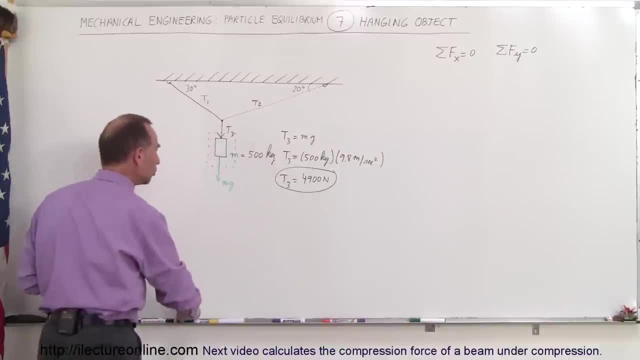 that into the components and we note that that will be equal to 4900 Newtons in a negative direction. but for tension 1 and tension 2, realizing that that tension- one, relative to this point where everything is connected- will be acting in this: 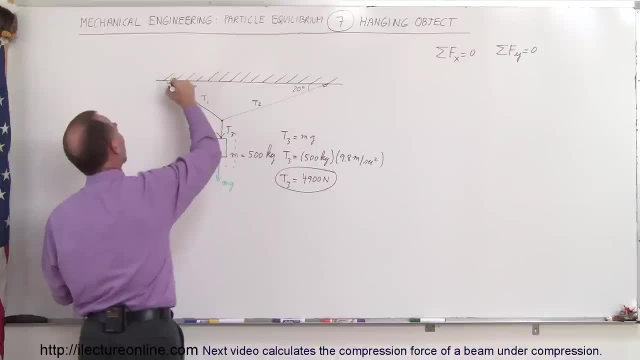 direction. Tension two will be acting in this direction. So these are the directions of tension one and tension two. So to find the components for tension one that would be equal to this component right here and this component right here. So this would be tension one in the y. 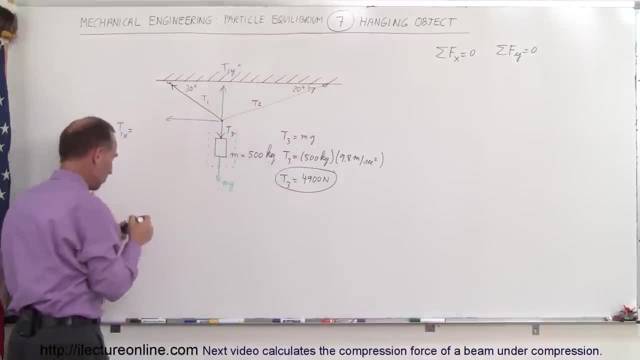 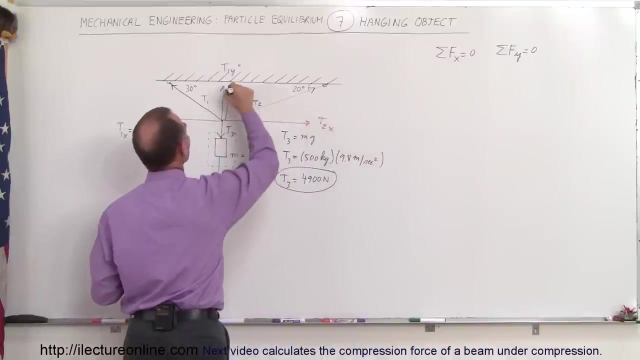 direction, and this would be tension one in the x direction. We'll find out in just a moment what those are equal to Using a different color, and let's use brown here. Here we can see that this would be tension two in the x direction, and this here would be tension two in the y. 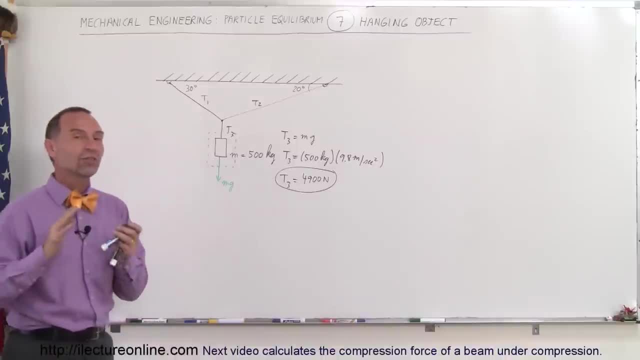 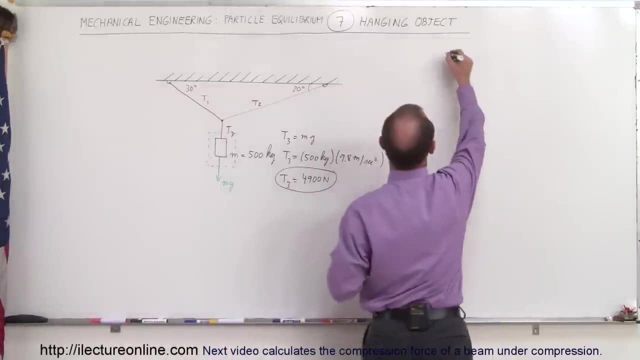 two components of each of the forces, because, again, it's a situation, it's an, it's a problem where everything is in equilibrium. and if, if everything is in equilibrium, we know that the sum of the forces in the x direction must add up to zero and the sum of the 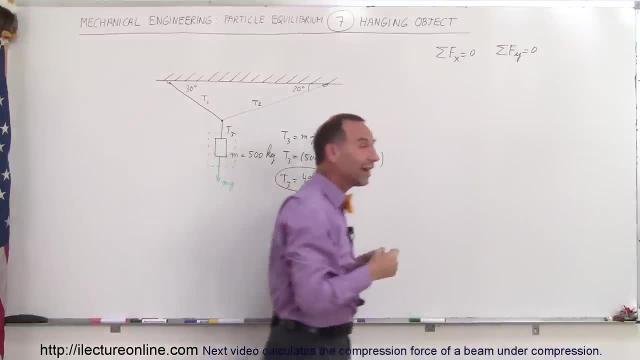 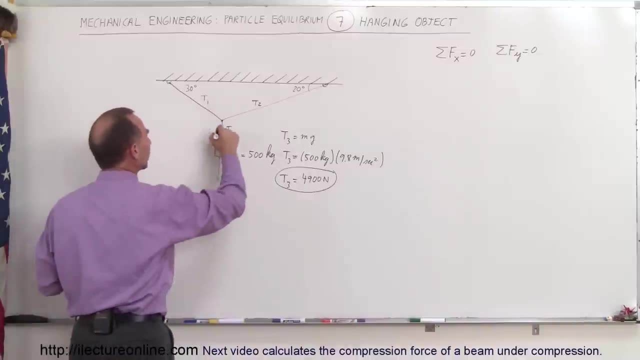 forces in the y direction must add up to zero, which means we need to find the x and y components of each of the forces there. Now notice: of course tension 3 will be acting in a downward direction. there's only one component, so we don't have to divide that into the components, and we note that. 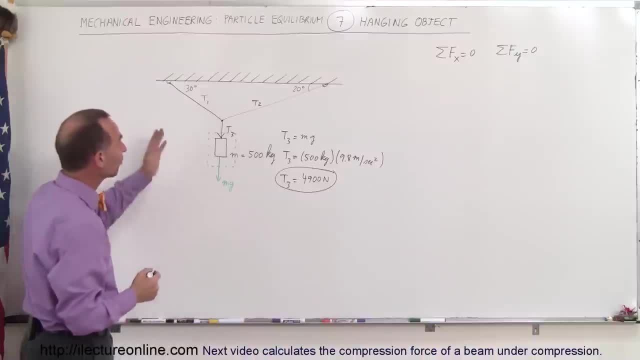 that will be equal to 4900 newtons in a negative direction. but for tension 1 and tension 2, realizing that tension 1, relative to this point where everything is going to be in equilibrium, and tension 2 will be acting in a downward direction. 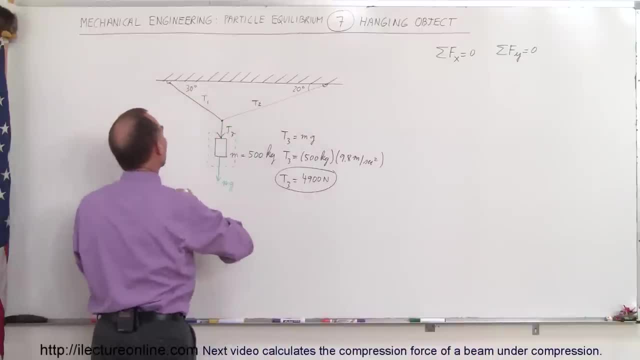 So these are the directions of tension 1 and tension 2. so to find the components for tension 1 that would be equal to this component right here and this component right here. so this would be tension 1 in the y direction and this would be tension 1 in the x direction. we'll find out in. 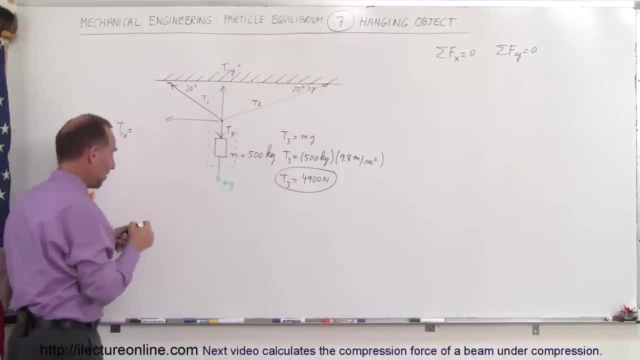 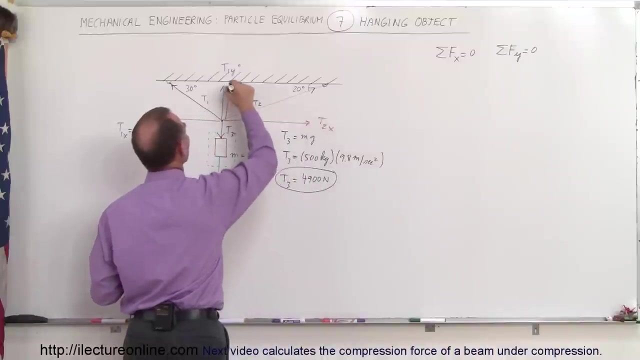 just a moment what those are equal to: Using a different color, and let's use, let's use- brown here. here we can see that this would be a negative component, and this would be a negative component and this would be tension 2 in the x direction, and this here would be tension 2 in the y direction. so 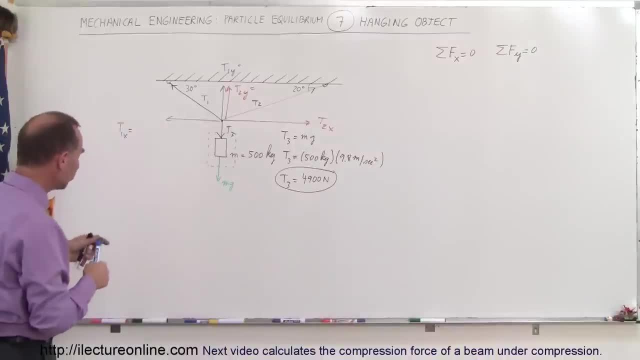 we have to find all four components. so to find tension 1 in the x direction, we need to find the angle. notice that this angle here and this angle would be the same right. so these are alternate interior angles. so this is 30 degrees, and then this here: if this is 20 degrees and this is 20, 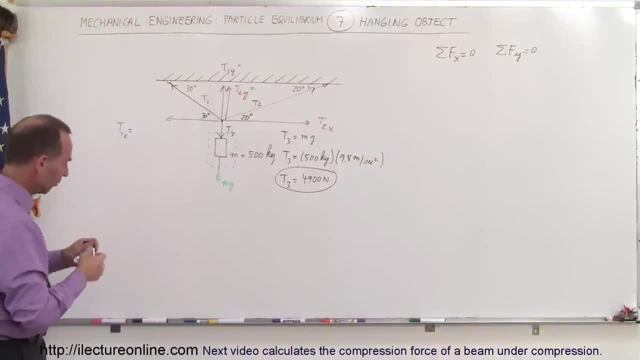 degrees as well. those are alternate interior angles. so here we can see that t1- x will be equal to t1. that would be the hypotenuse t1 times the cosine of 30 degrees, because that's the adjacent angle relative to this force right here. t1 in the y direction, that would be the opposite component. 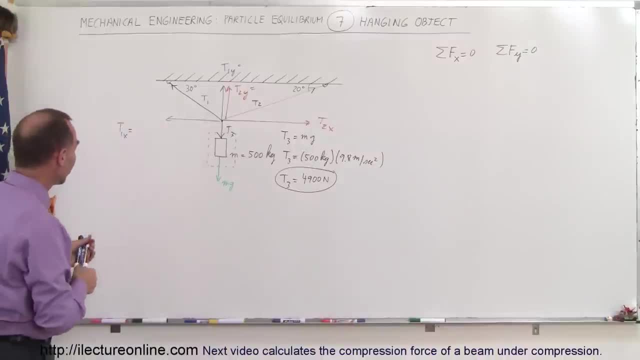 direction. So we have to find all four components. So to find tension, one in the x direction, we need to find the angle. Notice that this angle here and this angle would be the same right. So these are alternate interior angles. So this is 30 degrees and then this here. if this is, 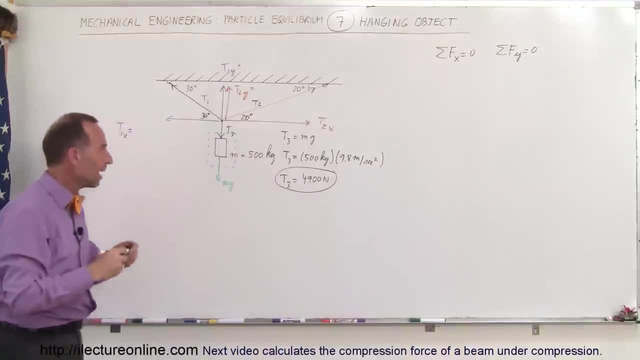 20 degrees and this is 20 degrees as well. those are alternate interior angles. so here we can see that t1- x will be equal to t1. that would be the hypotenuse t1 times the cosine of 30 degrees, because that's the adjacent angle relative to this force right here. t1 in the y direction, that 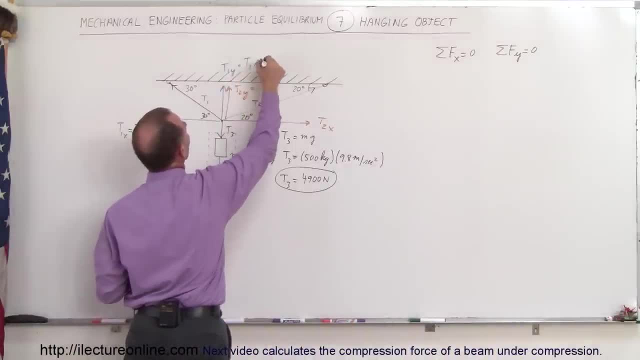 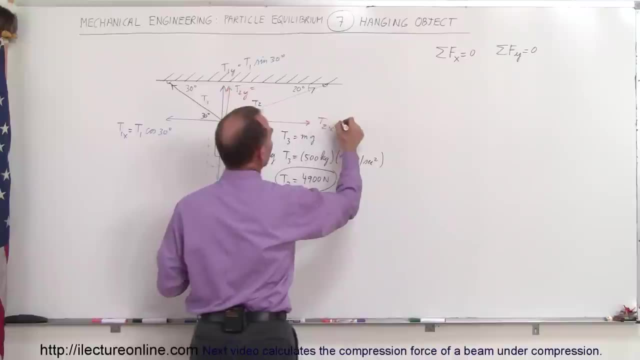 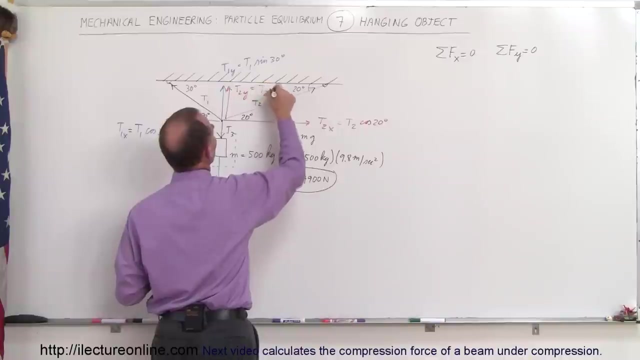 would be the opposite component. so this would be equal to t1 times the sine of 30 degrees. we can do the same for t2. t2 in the x direction would be equal to t2 times the cosine of 20 degrees, and t2 in the y direction would be t2 times the sine of 20 degrees. all right, since we don't know. 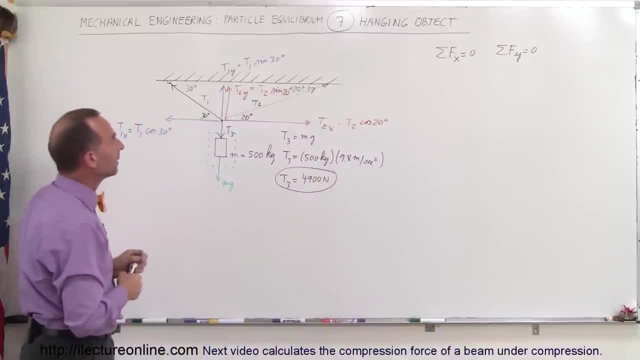 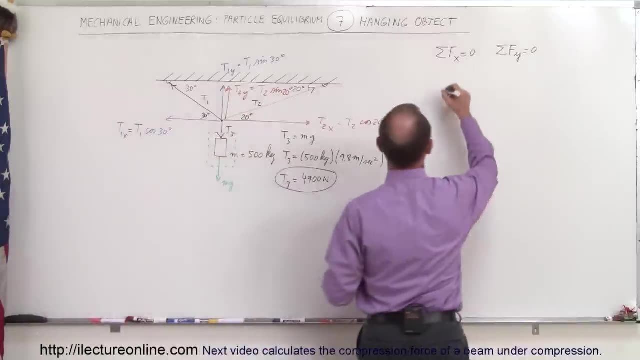 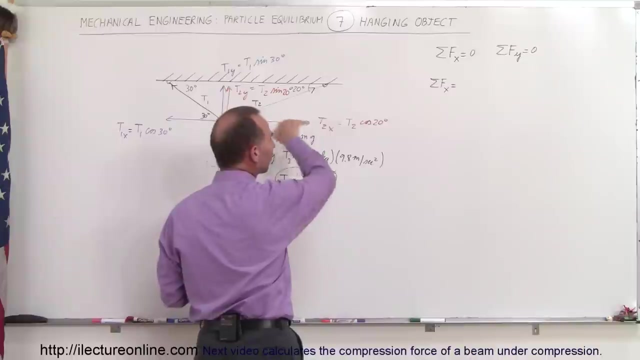 what those forces are. we just leave it like that and then we can go ahead and plug that into our two equations right up there. so in the x direction some of the forces in the x direction is equal. to notice that t2 x is in the positive x direction. so that would be a positive t2 x and 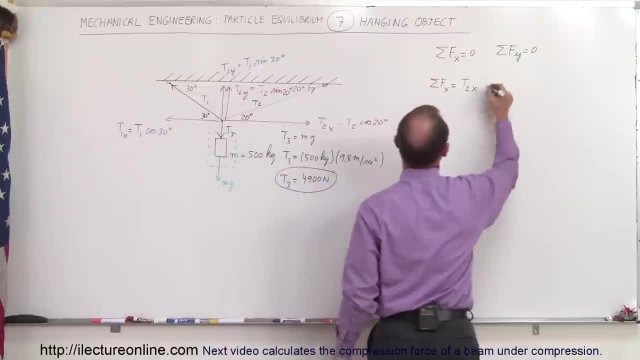 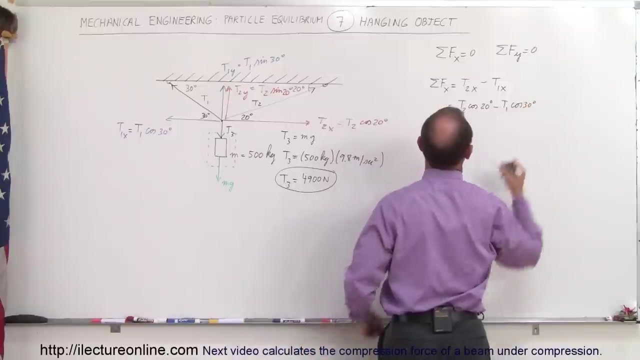 t2 in the y direction. t1 in the y direction is negative, so it'd be minus t1 x, and so that would be equal to t2 times the cosine of 20 degrees, minus t1 times the cosine of 30 degrees. so let's. 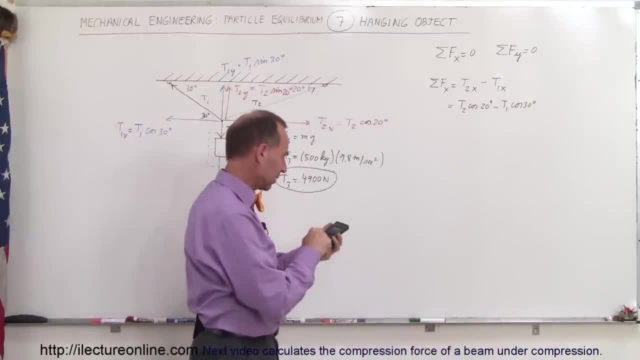 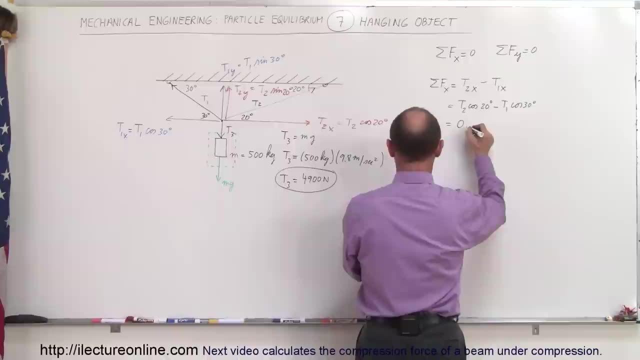 go ahead and figure out what those are. so 20 take the cosine of that, that is equal to 0.9397. so it would be equal to 0.9397 times t2 minus take the cosine of 30, that would be 0.8660 times t1 and that would be equal to 0, because the sum 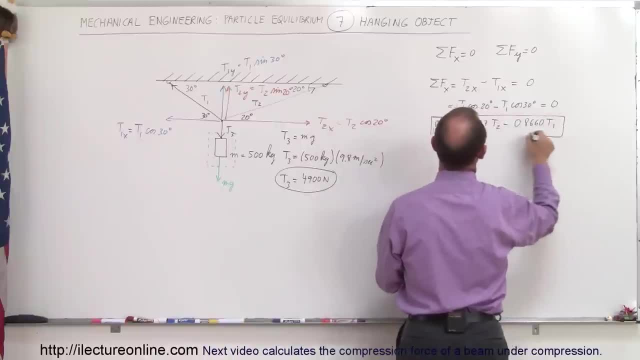 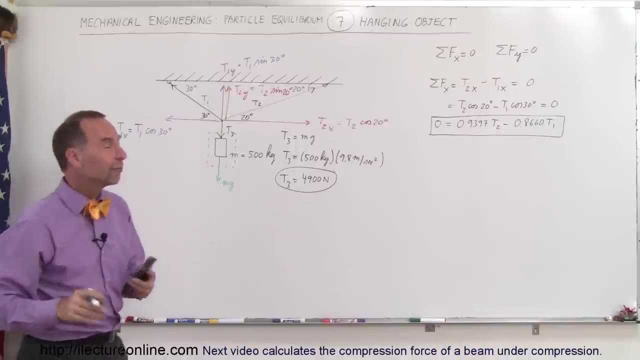 of the force in the x direction would have to add up to 0. so there's my first equation, the one i got from the summation of the forces in the x direction. we'll now do the same for the force in the y direction. so the sum of the 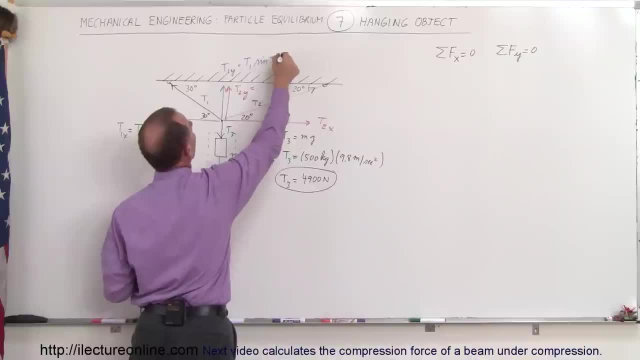 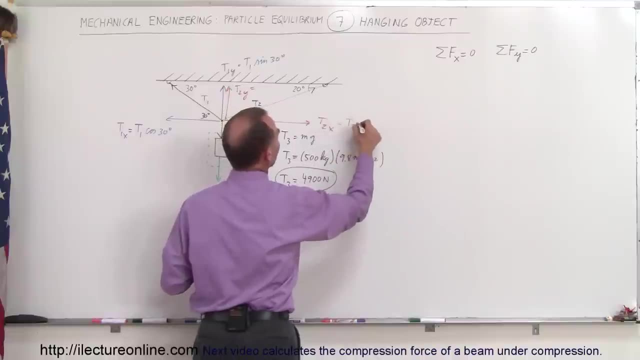 so this would be equal to t1 times the sine of 30 degrees. we can do the same for t2. t2 in the x direction would be equal to t2 times the cosine of 20 degrees, and t2 in the y direction would be t2. 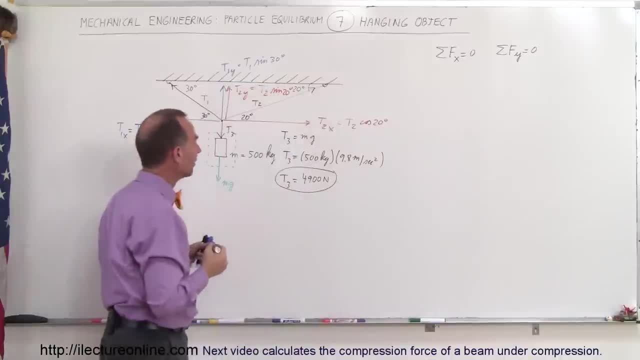 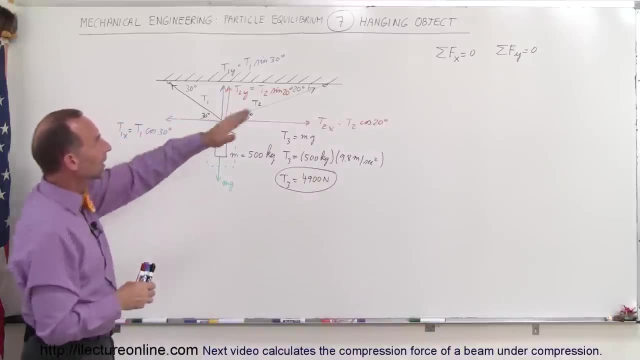 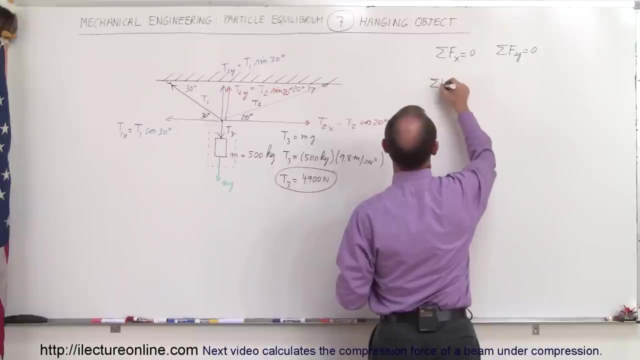 times the sine of 20 degrees. all right, since we don't know what those forces are, we just leave it like that and then we can go ahead and plug that into our two equations right up there. so in the x direction, sum of the forces in the x direction is equal. to notice that t2x is in the positive. 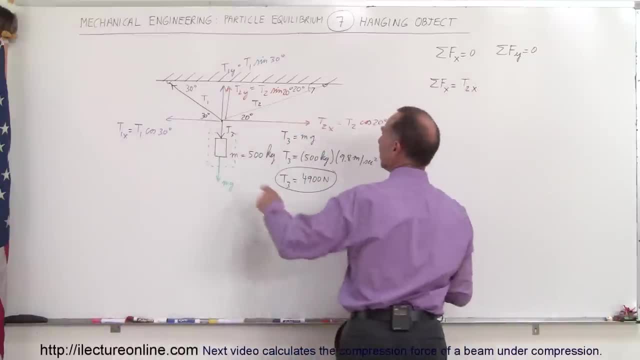 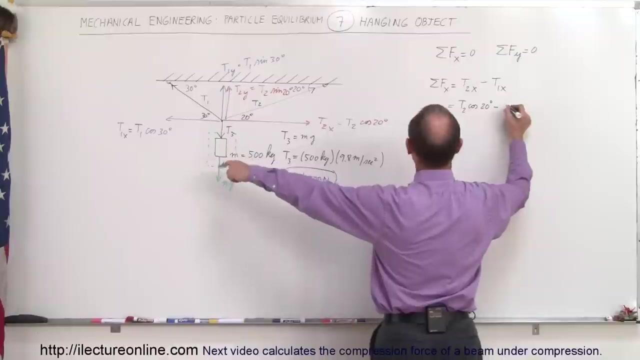 x direction, so that would be a positive t2x and t2 in the y direction. t1 in the y direction is equal to minus t1 x, and so that would be equal to t2 times the cosine of 20 degrees, minus t1 times the cosine of 30 degrees. so let's go ahead and figure out what those are. 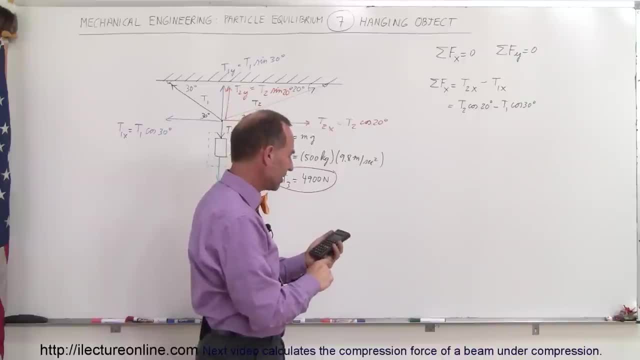 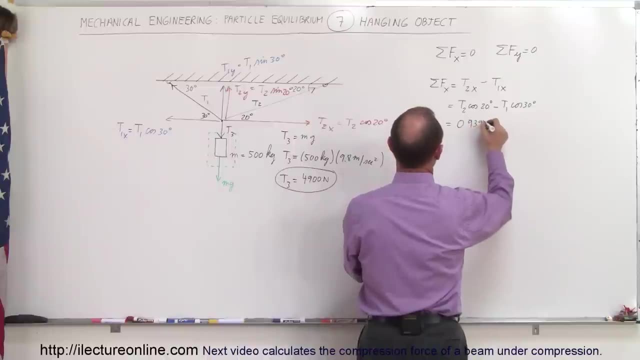 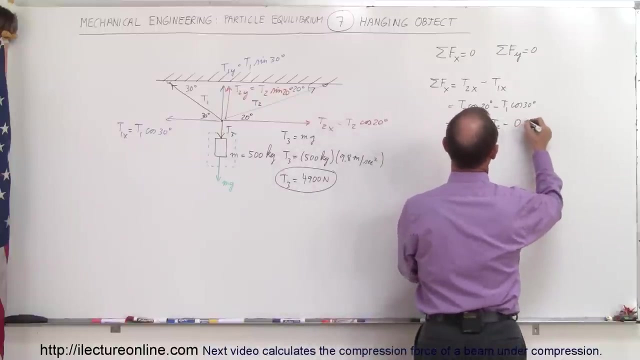 so 20. take the cosine of that, that is equal to 0.9397. so it would be equal to 0.9397 times t2 minus take the cosine of 30, that would be 0.8660 times t1 and that would be equal to 0, because the 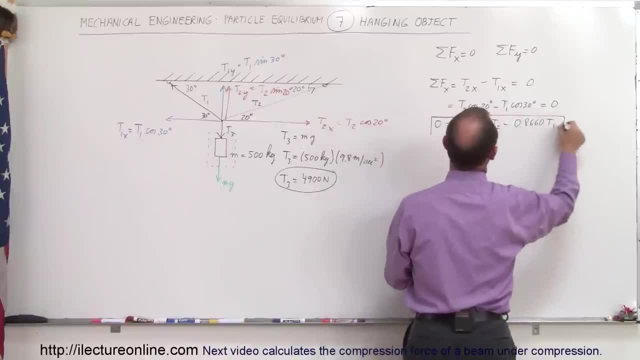 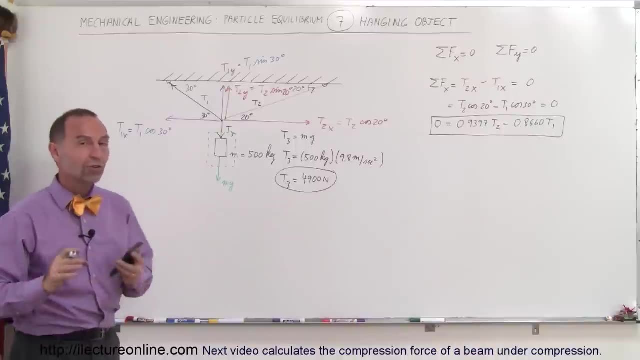 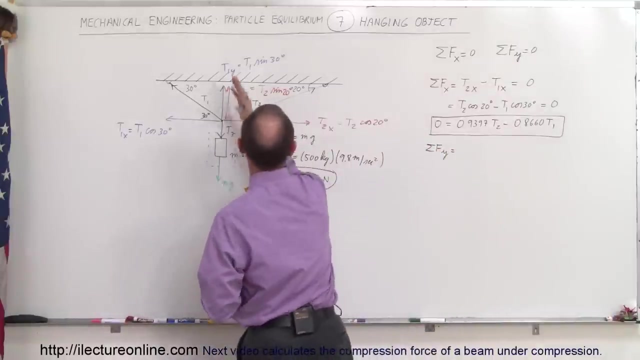 sum of the force in the x direction would have to add up to 0.. so there's my first equation, the one i got from the summation of the forces in the x direction. we'll now do the same for the force in the y direction. so the sum of the forces in the y direction is equal to. we have this force right here. 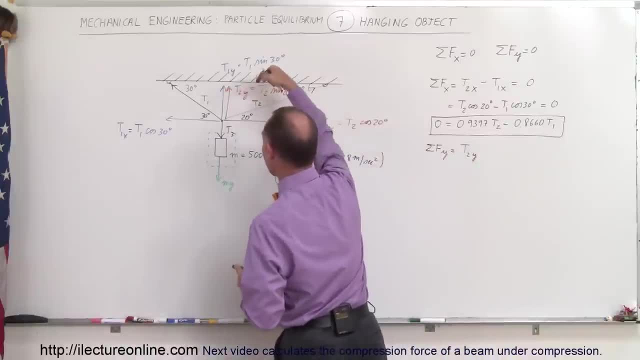 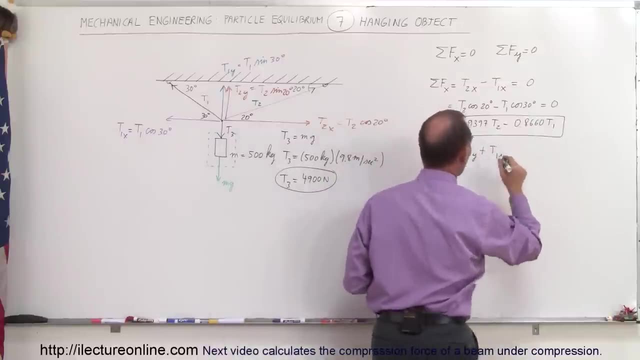 t2 in the y direction. that's positive. and do we have anything in the negative there? oh, we have another one, t1 y. so we plus t1y, they're both. both components are in the positive y direction. and then we of course have the minus 4900 newtons in the y direction, which is the weight of the object. 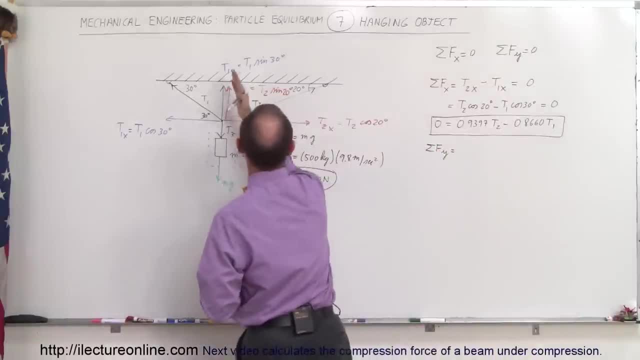 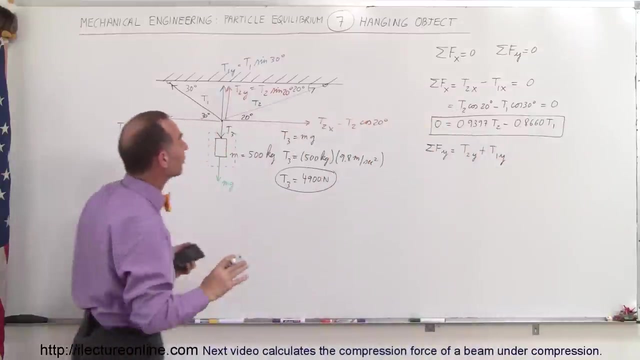 forces in the y direction is equal to. we have this force right here, which is t2 in the y direction. that's positive. and do we have anything in the negative there? oh, we have another one, t1 y, so it would be plus t1 y. they're both. both components are in the positive y direction. and then we of 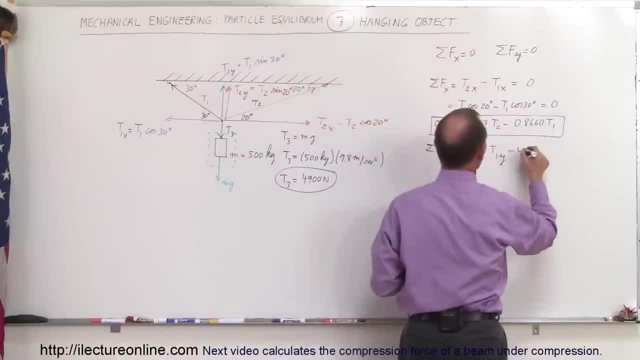 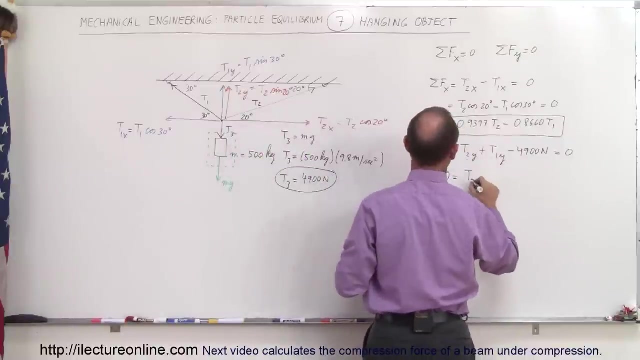 course have the minus 4900 newtons in the y direction, which is the weight of the object. all right, and plug in what those are equal to. so that would be equal to 0. so 0 is equal to t2 y. t2 y would be t2 times the sine of 20 degrees, plus t1 times the 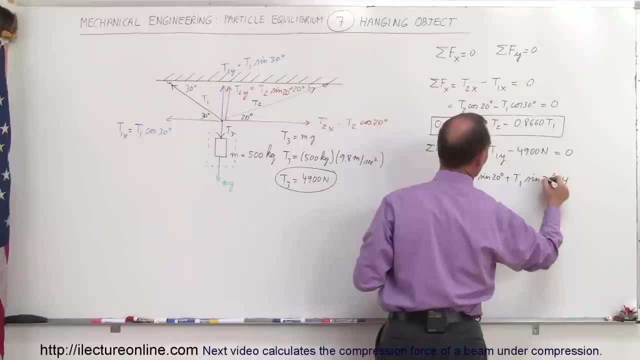 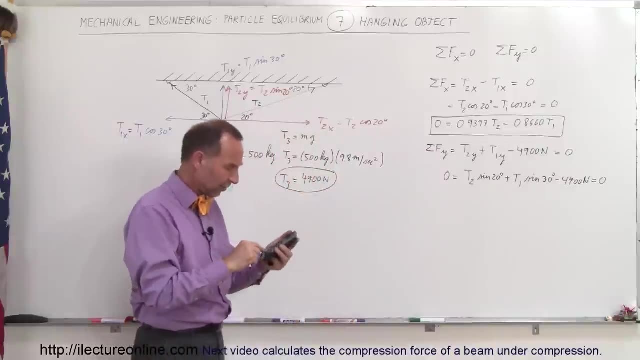 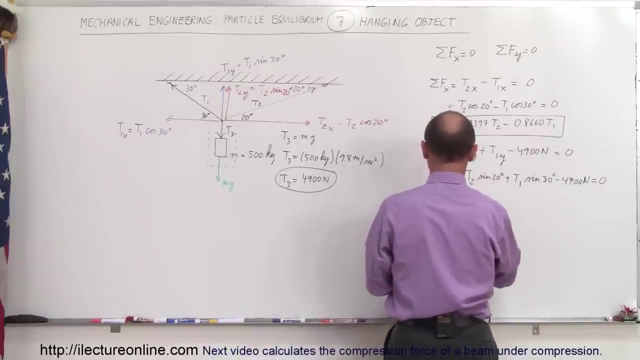 sine of 30 degrees minus 4000, that's a 3 minus 4900 newtons equal 0. all right, finding out what the sine of 20 is. so the sine of 20 would be 0.3420. so 0 equals 0.3420 times t2, plus the sine of 30 degrees is: 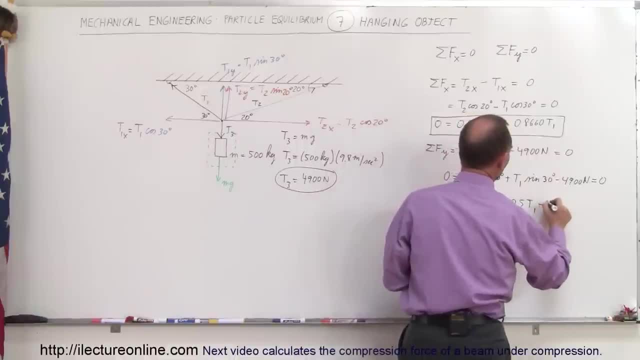 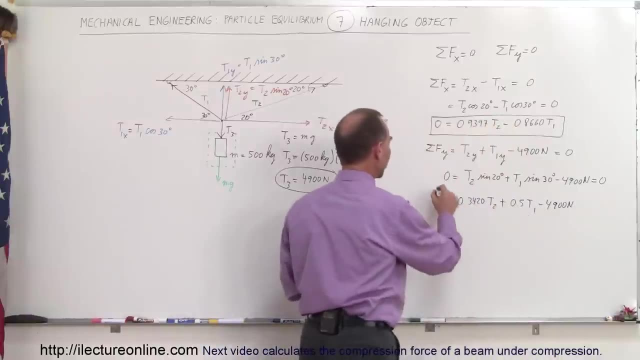 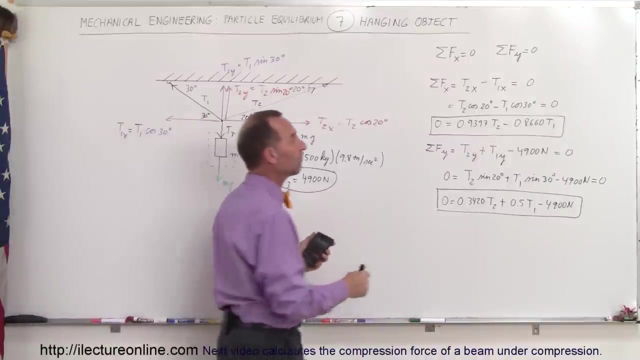 one half, so 0.5 times t1 minus 4900 newtons equals 0. i already have equals 0. all right, so there's my second equation. now those two equations have two unknowns. they both have a known t1 and t2. t1 and t2. so we have to solve one of the equations for one of the 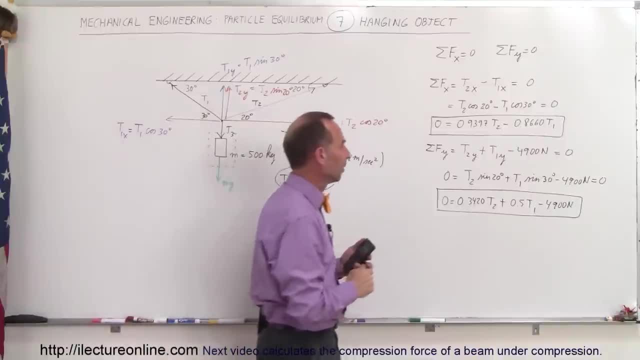 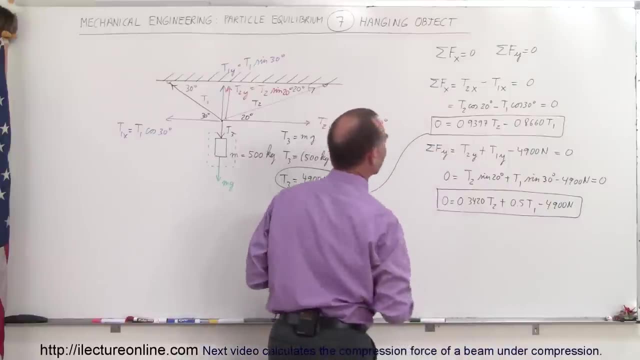 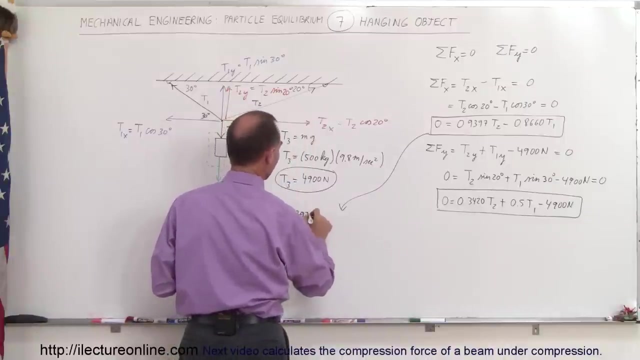 variables and then substitute that into the second equation. so what would be the easiest thing to do? well, let's go ahead, doesn't really matter. so let's take this equation right here and solve for t2 in terms of t1, so we have 0.9397 t2. well, if i put this on the other side, it becomes positive. so it. 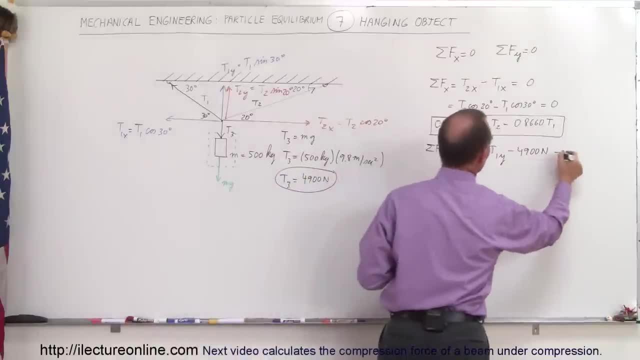 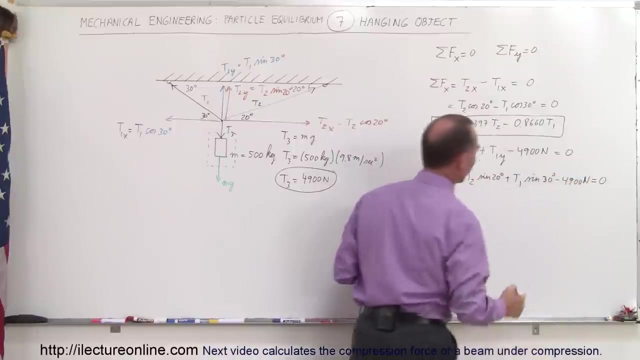 all right, and plug in what those are equal to. so that would be equal to zero. so zero is equal to t2 y. t2y would be t2 times the sine of 20 degrees plus t1 times the sine of 30 degrees minus four thousand, that's a three minus four thousand nine hundred newtons. equal zero. all right. 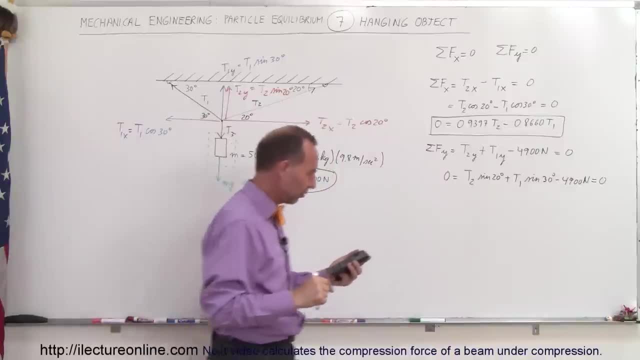 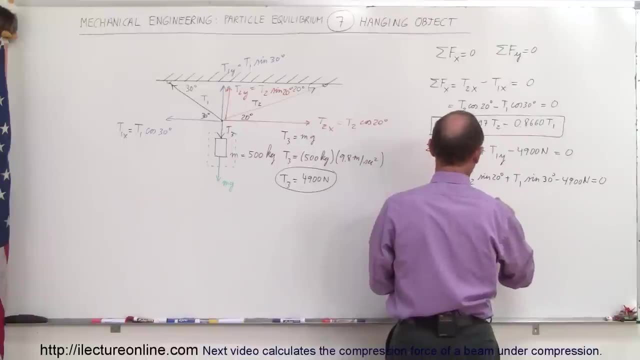 find out what the sine of 20 is. so the sine of 20 would be 0.3420. so 0 equals 0.3420 times t2, plus the sine of 30 degrees is one half. so 0.5 times t1 minus 4900 newtons equals zero. i already 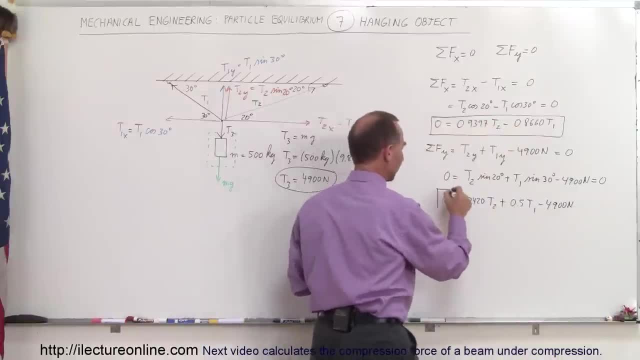 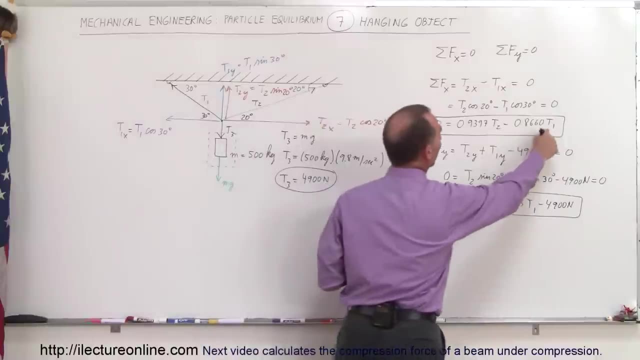 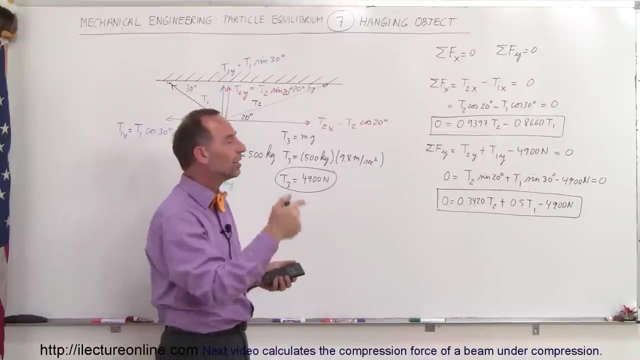 have equals there. all right, so there's my second equation. now those two equations have two unknowns. they both have a known t1 and t2, t1 and t2. so we have to solve one of the equations for one of the variables and now substitute that into the second equation. 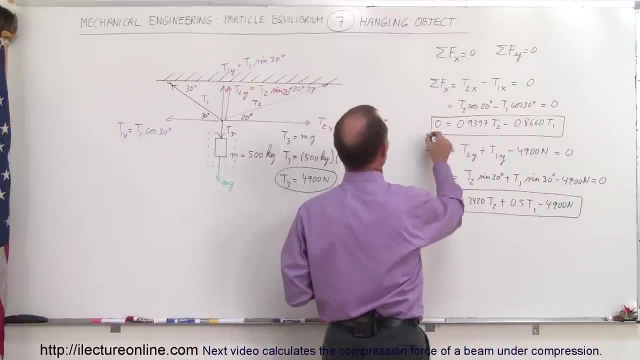 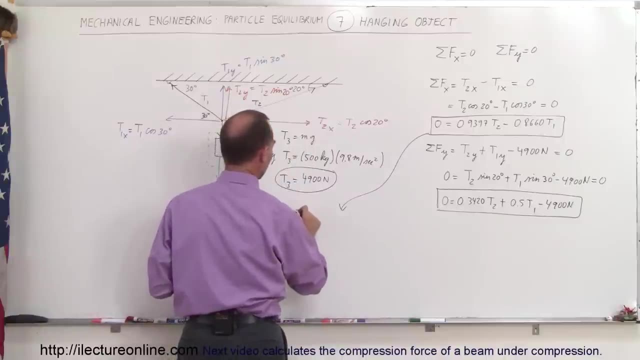 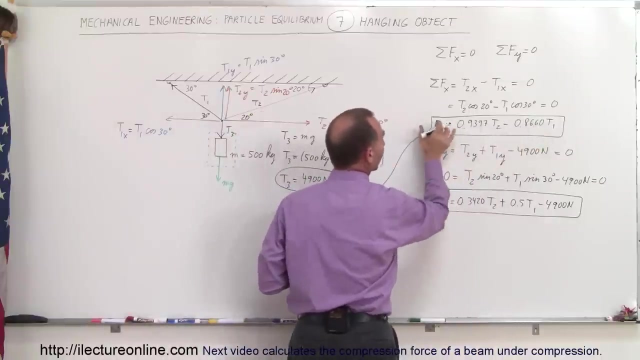 so what would be the easiest thing to do? well, let's go ahead, doesn't really matter. so let's take this equation right here and solve for t2 in terms of t1. so we have zero point nine, three, nine, seven, t2. well, if i put this on the other side, it becomes positive. so it would be equal to a positive. 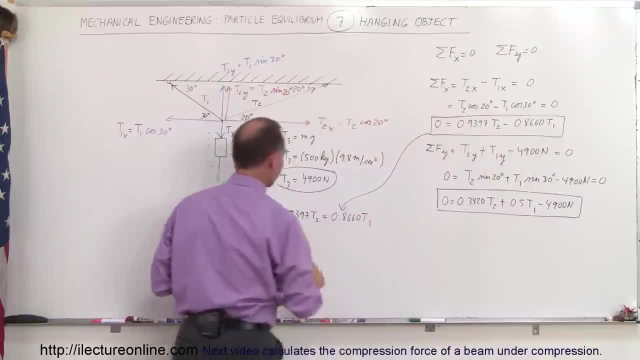 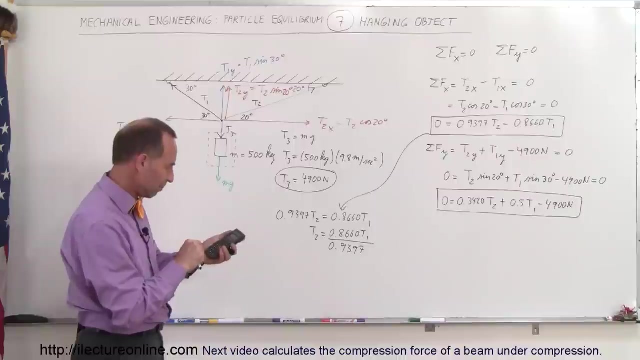 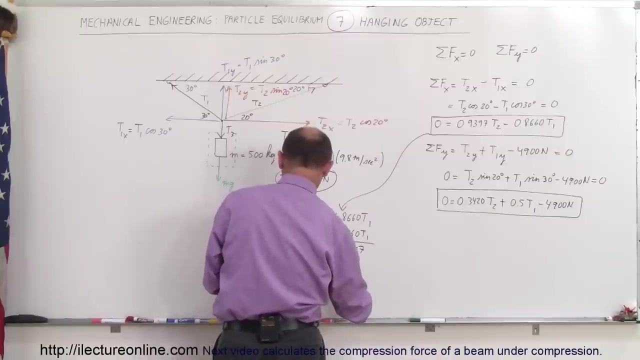 zero point eight, six, six zero t one. therefore, t two is equal to zero point eight six six zero t one. the t two is equal to zero point nine, three, nine, seven. so point eight six six divided by point nine, three, nine seven equals. so i know that t2 is equal to zero point nine two one, six times t1, so that 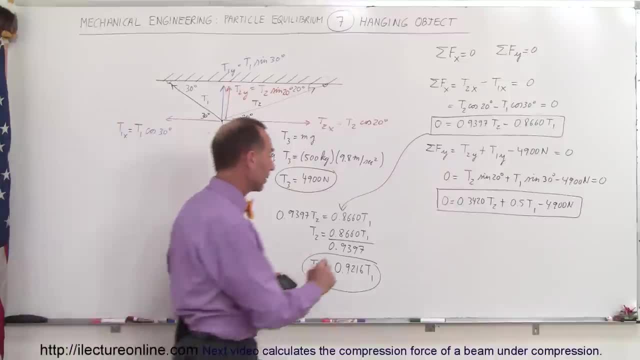 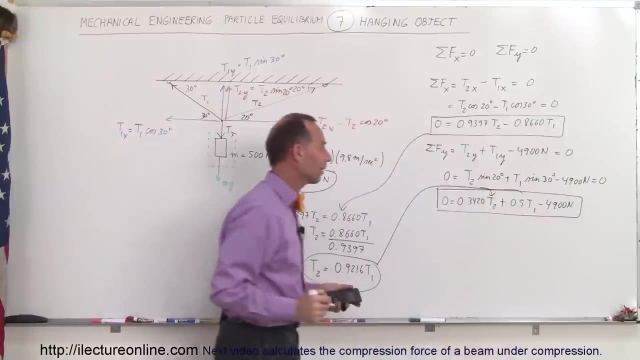 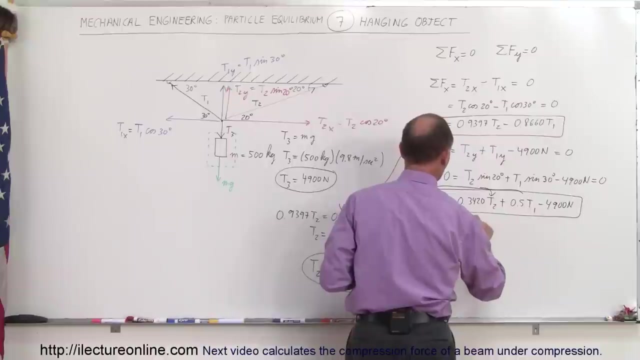 allows me to find what t2 is in terms of t1, then i can go ahead and plug that into my equation right right here. okay, a little too far, so i'm going to go ahead and plug that into t2 in my second equation. so that means that zero is equal to zero. point three, four, two, oh times. t2 is now going to be. 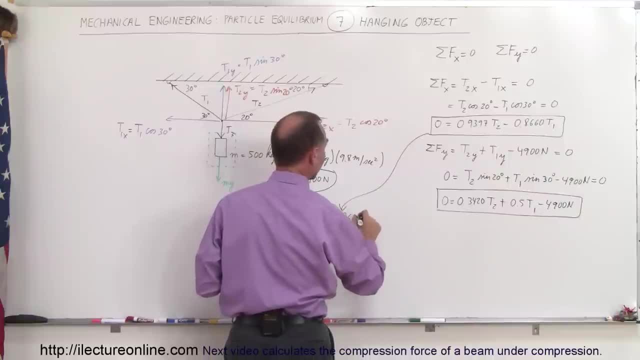 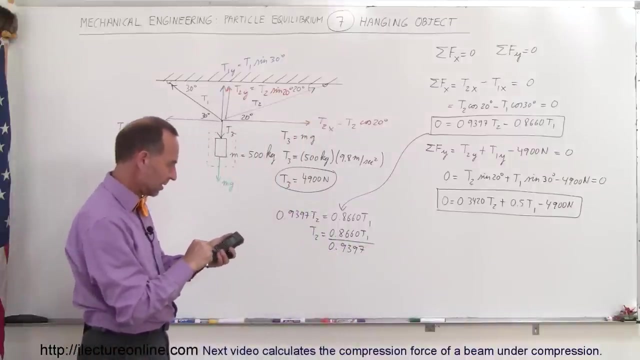 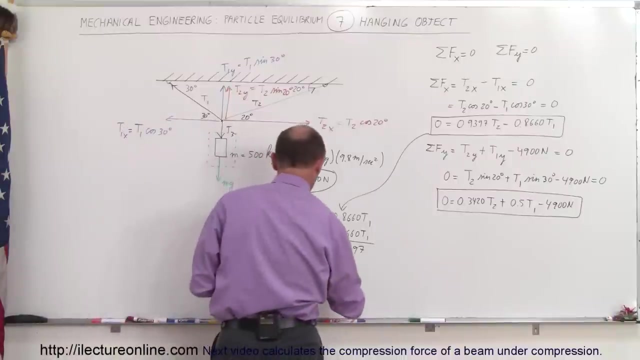 will be equal to the positive 0.8663 t1. therefore, t2 is equal to 0.860 t1 divided by 0.9397, so .866eplD by .9397. so i know that t2 is equal to 0.9216 times 0.866 by 9367. that will, Mary àe Nabb, occurring zero sound. 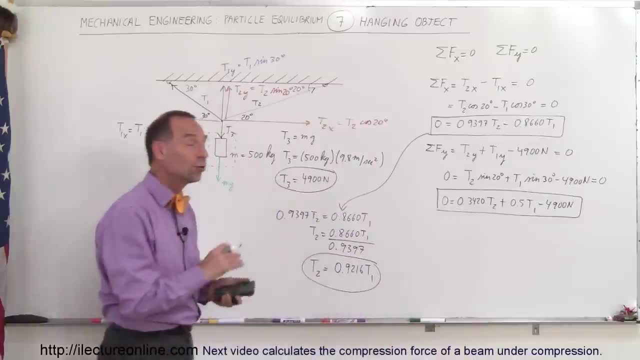 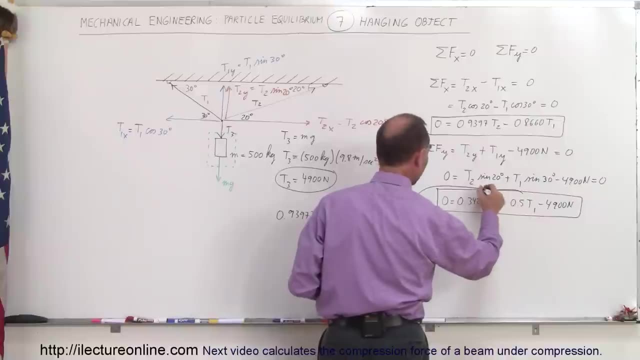 times t1. so that allows me to find what t2 is in terms of t1. then i can go ahead and plug that into my equation right right here. okay, went a little too far, so i'm going to go ahead and plug that into t2 in my second equation. so that means that zero is equal to 0.3420 times t2 is now going. 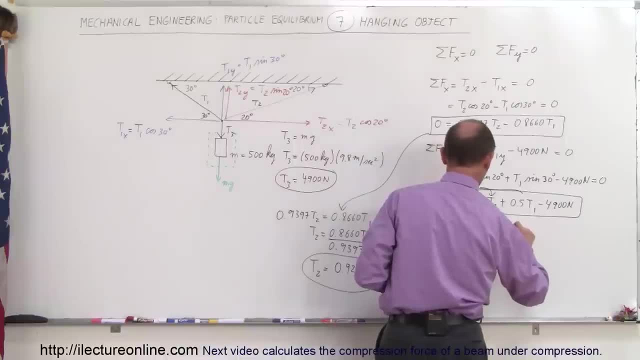 to be 0.9216 t1 plus 0.5 t1 minus 4900. all right, now i have to solve that equation. for t1, which means i'm going to take the 4900 newtons that are negative to the other side, becomes: 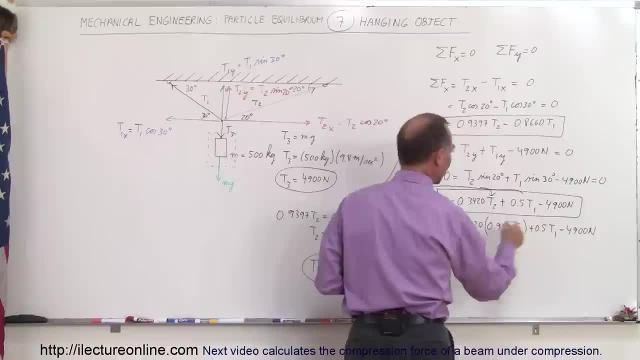 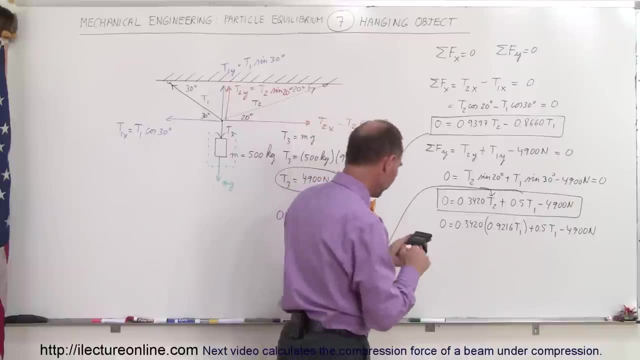 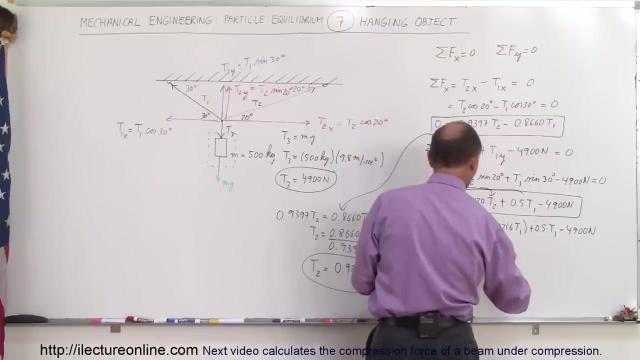 positive. flip the whole equation around, multiply this to add it together, and what do we get? so times 0.342 equals. so that gives me 0.3152 times t1 plus 0.5 t1 is equal to 4900 newtons. so i went ahead and multiplied. 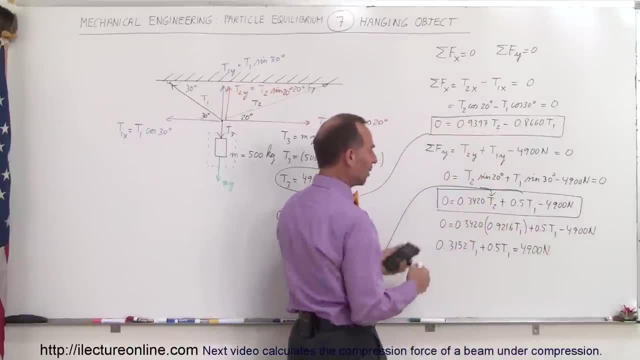 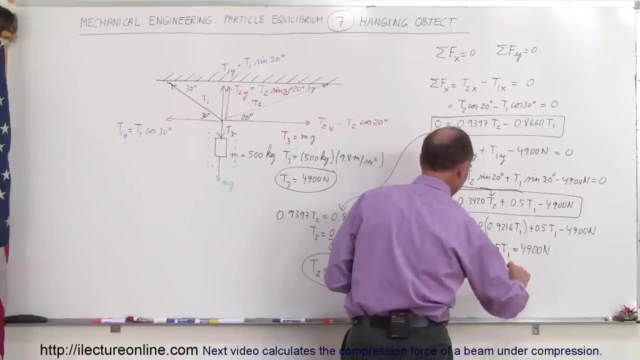 this together and moved the 4900 newtons to the other side. flip the equation around so this becomes 0.8152. t1 equals 4900 newtons and finally i divide both sides by the coefficient of t1, so plus 0.5. 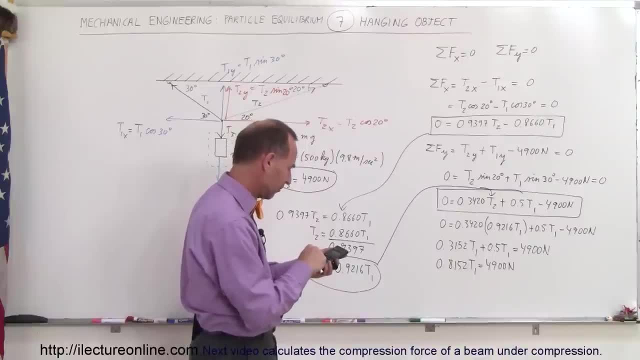 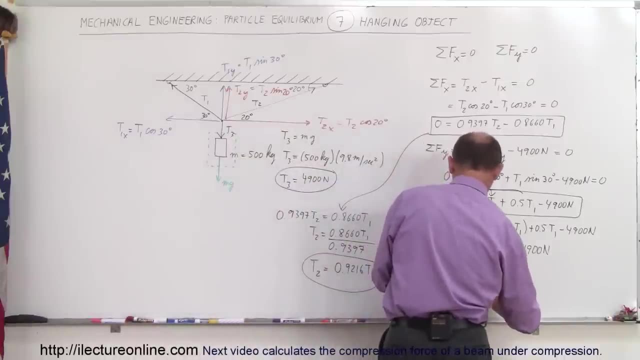 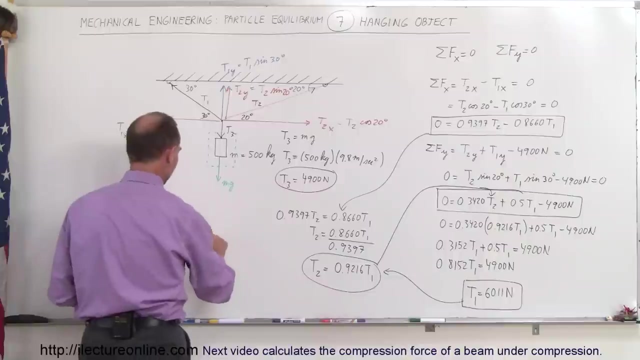 equals and take the inverse times 4900 equals. so that means that t1 is equal to 6000 and 11 newtons. now that i have t1, i can plug that back into my other equation to find t2. so t2 is going to. be equal to 0.9216 times t1. and now i need to find t1, so that is TII in our second equation. if i plug t1 into my second equation, well i can get. takes or gives us 0.92 my 6 times 2 once. 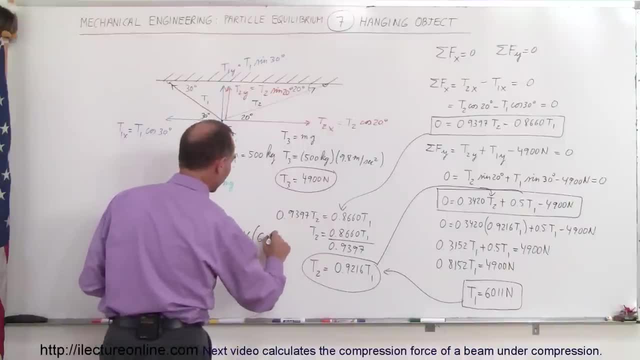 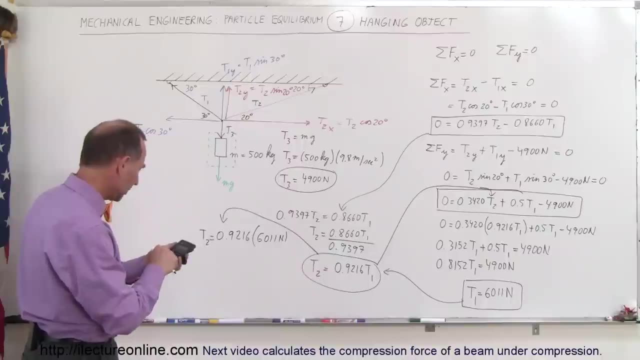 다음에 0.9216. my second equation was 0.9226. this is ± 0.956, 5 times ± 0.956, which i have, T1 is 6,011 newtons, so this becomes this equation right there. so times 0.9216 equals. 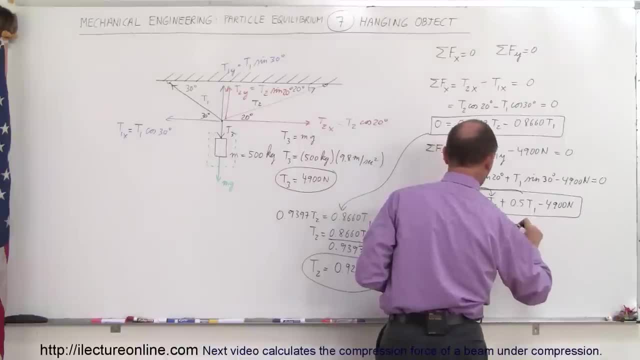 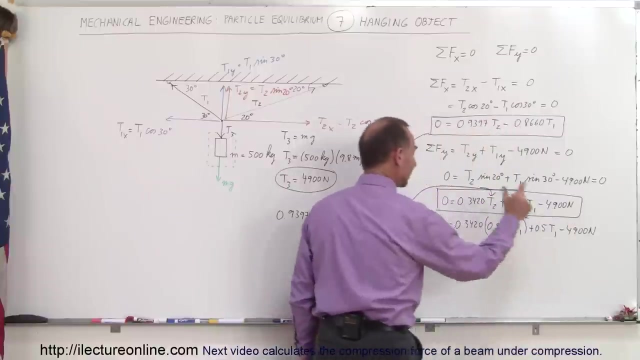 zero point nine, two one, six t one plus zero point five t one minus forty nine hundred. all right, now i have to solve that equation for t one, which means i'm going to take the forty nine hundred newtons that are negative to the other side, becomes positive. flip the whole equation around, multiply this to add it together. 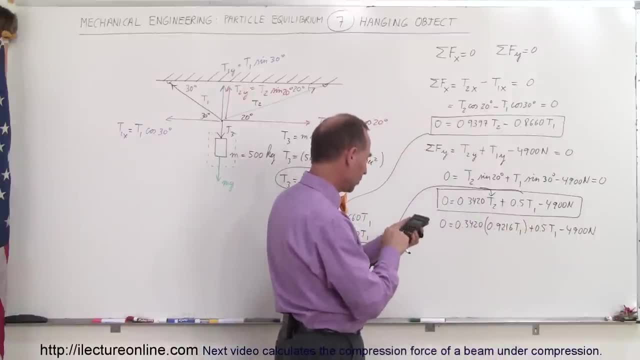 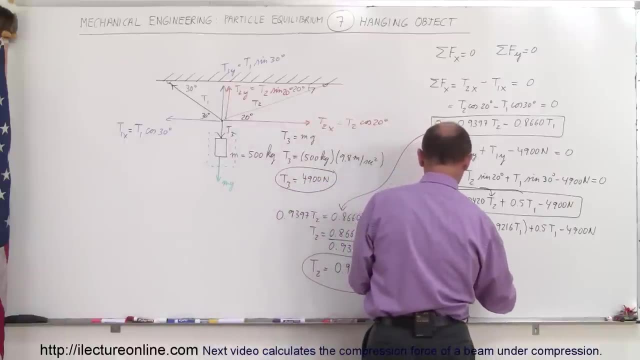 and what do we get? so times 0.342 equals. so that gives me 0.3152 times t1 plus 0.5 t1 is equal to 4900 newtons. so i went ahead and multiplied this together and moved the 4900 newtons to the other. 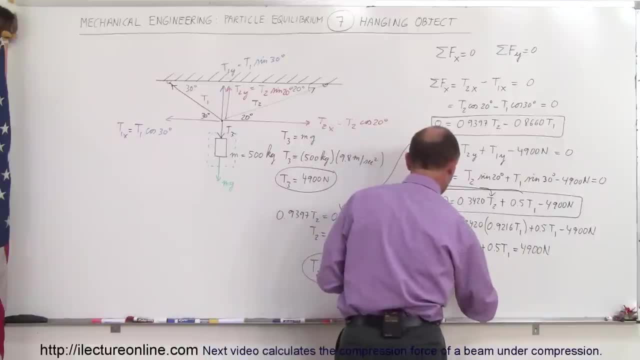 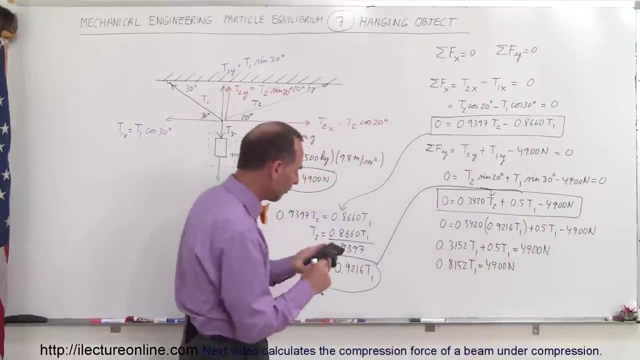 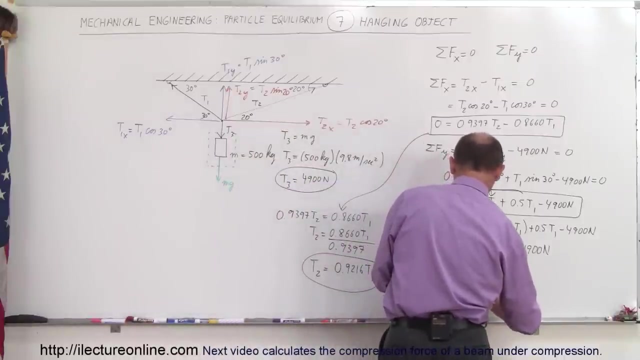 side. flip the equation around so this becomes 0.8152. t1 equals 4900 newtons. and finally i divide both sides by the coefficient of t1, so plus 0.5 equals, and take the inverse times 4900 equals, so that means that t1 is equal to six thousand and eleven newtons. 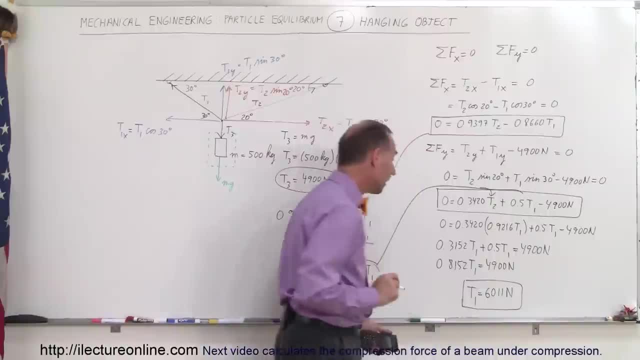 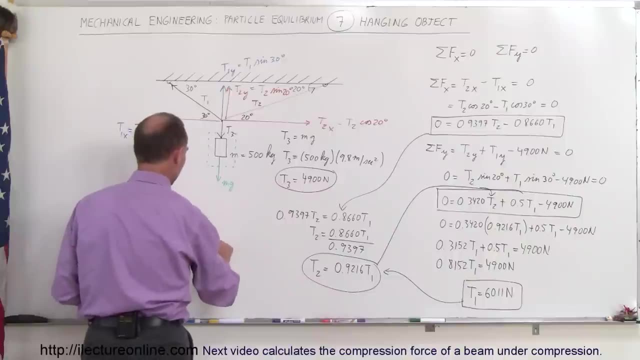 so now that i have t1, i can plug that back into my other equation to find t2. so t2 is going to be equal to 0.9216 times t1, and t1 is six thousand and eleven newtons. so this becomes this equation. 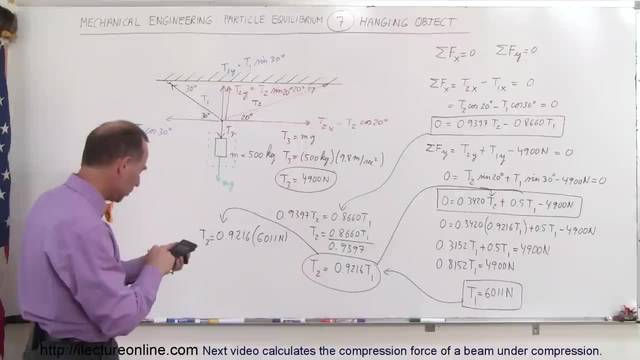 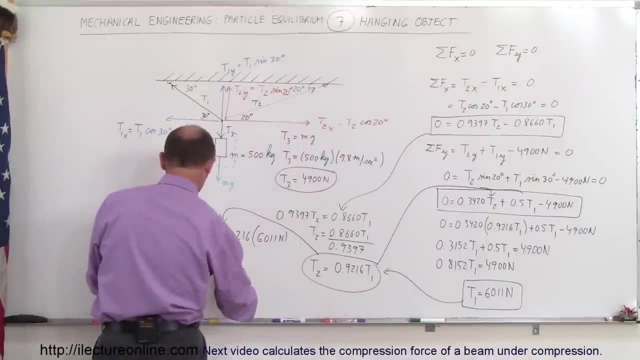 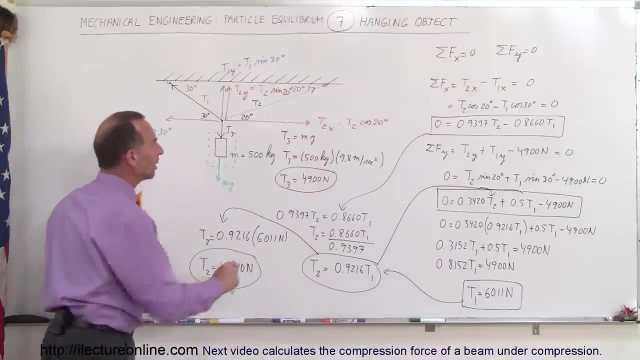 right there. so times 0.9216 equals, and so that means t2 is equal to 5, 5 540 newtons. so t3, 4900 newtons. t2, which is this one right here, that would be t2, is 5 540 newtons. 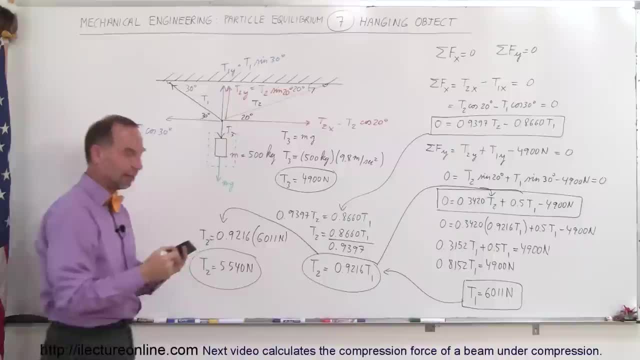 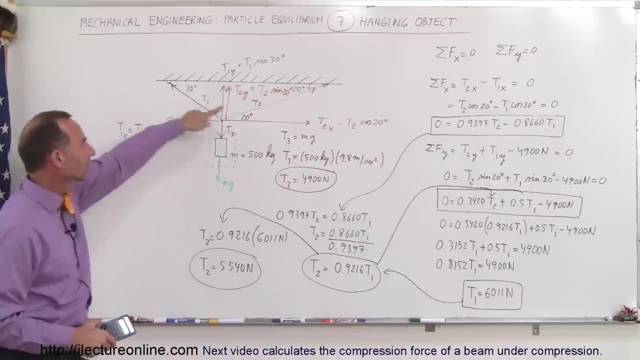 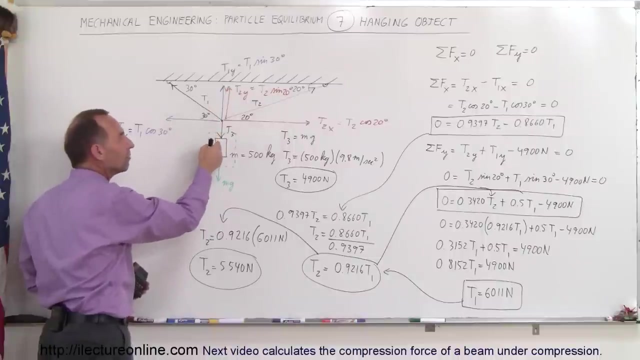 and t1 is six thousand and eleven newtons. that's kind of an interesting result. so why does t1 have more of more tension than t2? well, notice that the angle here is bigger and the angle here is smaller, which means that t1 carries more of the weight of this object than t2 does t2, however?